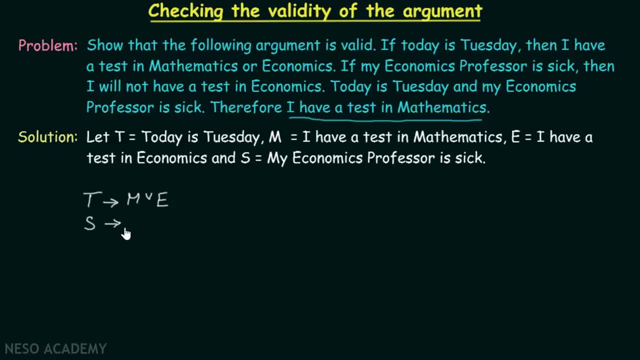 If my economics professor is sick, then I will not have a test in economics. Today is Tuesday and my economics professor is sick. Therefore, I have a test in mathematics. So this is our argument And what we need to check. We need to check the validity of this argument. 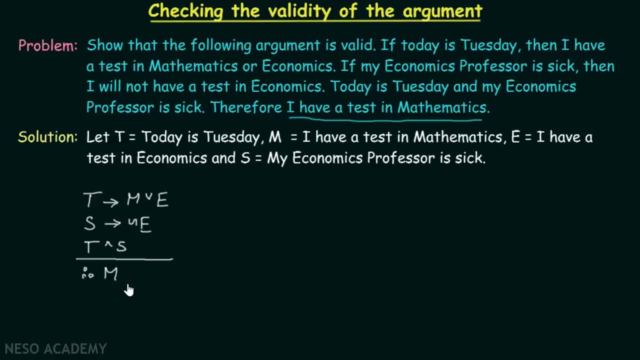 Is this argument is valid or not. There are definitely multiple ways to check the validity of the argument. One method is to check it by the rule of inference, But there is one more, better method which we can apply right now, And that method is considered to be. 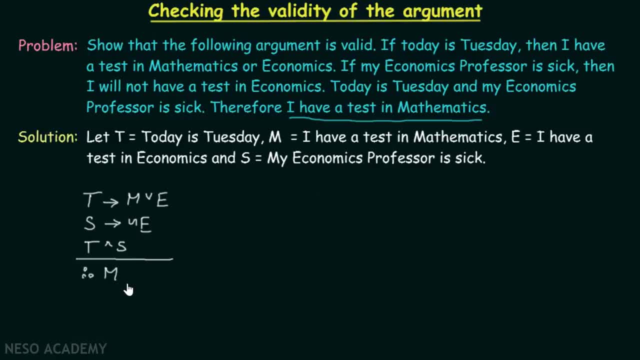 the fastest method among all. Let's use that method to prove the validity of this argument. According to that method, we need to make all these premises true and conclusion false. If we make all the premises true and conclusion false, then definitely this argument is an invalid argument. 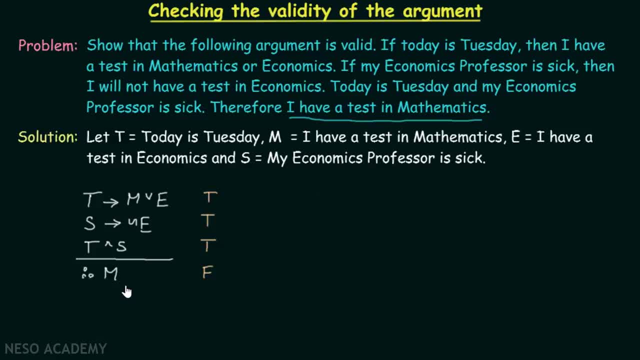 Right. But if we would not be able to make all the premises true and conclusion false, then without any doubt we can say that this argument is a valid argument. Okay, Let's try to make all premises true and conclusion false, As we need to make conclusion false. 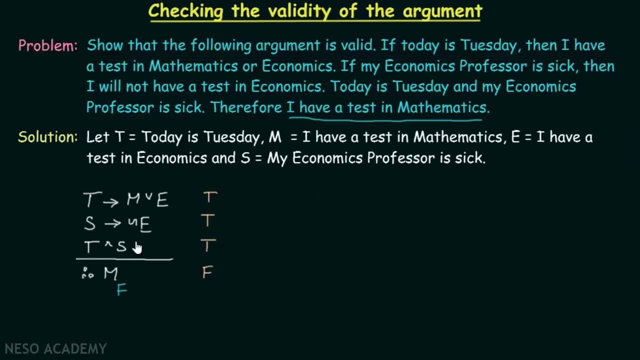 therefore, M has to be false. We need to make this premise true. This premise can be true only when, when T is true and S is true. This is the only way we would be able to make this premise true. If S is true. 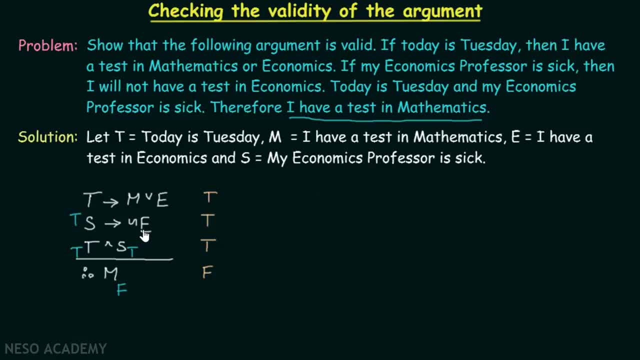 then not. E cannot be false. It has to be true Right, Therefore not E will be true. And if not E is true, then E becomes false Right. And we already know M is false and T is true. M is false and T is true. 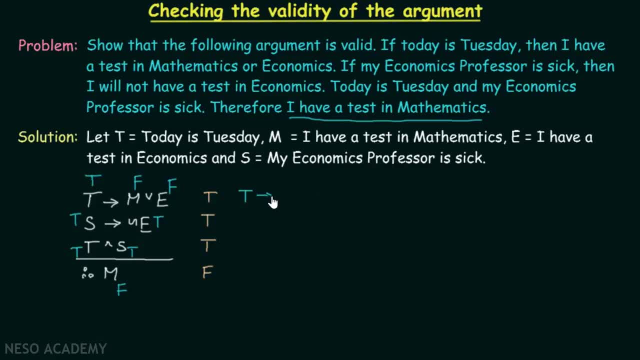 This particular premise is of the form: true implies false, Which is false. Right, We are successful in making this premise true, this premise true, this conclusion false. But we won't be able to make this particular premise true And due to this reason,